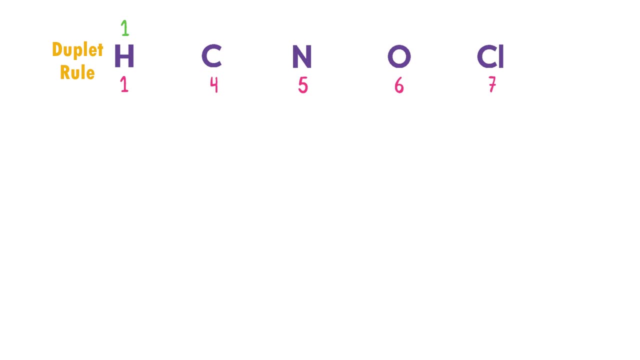 electron to complete its duplicate rule and get stability. There are already four electrons present in the valential of carbon, So it needs four more electrons to complete its octet rule and get stability. Similarly, nitrogen needs four electrons to complete its octet. 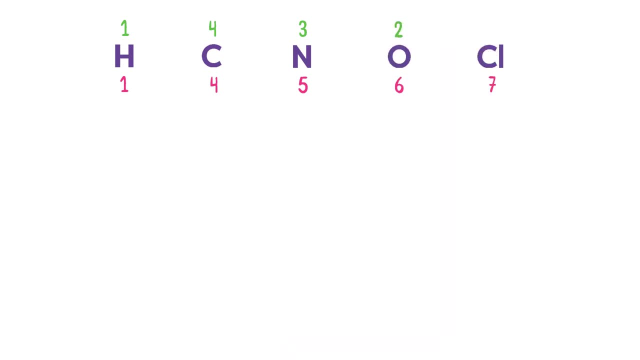 rule and get stability. So we know that oxygen needs three more electrons, Oxygen needs two more electrons and chlorine needs only one electron to complete its octet rule and get stability. Now let me draw the Lewis structure of these elements. Write the symbol. 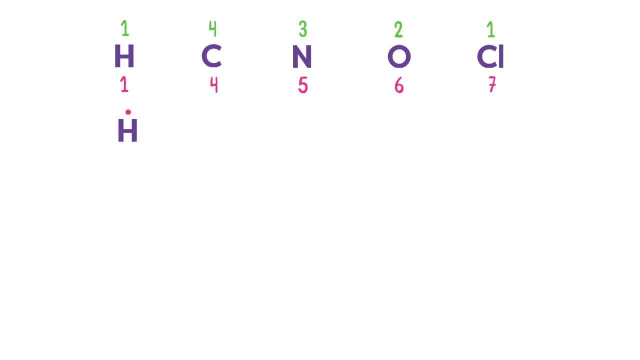 of hydrogen H and then put the dot on it. This dot represents the valence electron of hydrogen. Similarly, I write carbon and put four dots on it. I write nitrogen and put put 5 dots on it. I write oxygen and put 6 dots on it And finally I write chlorine. 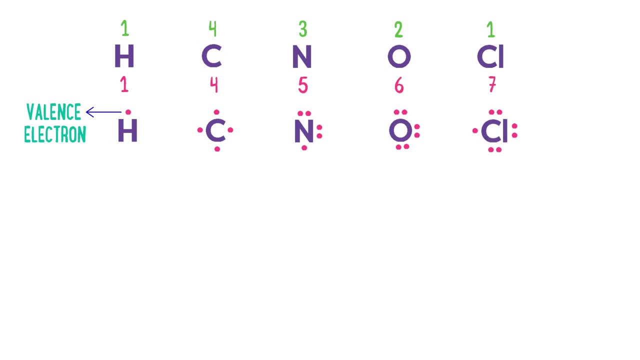 and put 7 dots on it. These are the Lewis structure of these elements. Now I will use these structures in order to draw the Lewis structure of any compound or molecule. For example, consider hydrogen molecule. Here H2 means that there are two atoms of hydrogen. 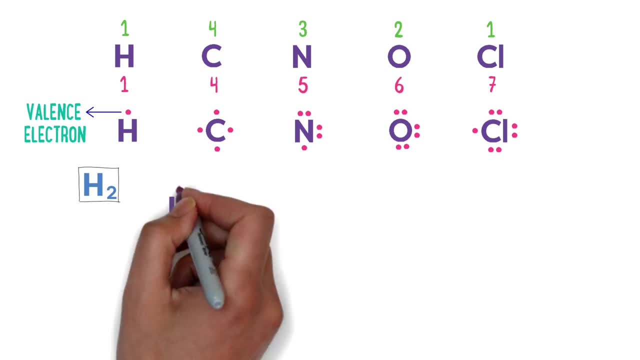 are present in this molecule. So I take two atoms of hydrogen. Now this single electron of this hydrogen atom and this single electron of this hydrogen atom are mutually shared. It means that two electrons, or one pair of electrons, is shared between these two hydrogen atoms and we get this structure. Remember that these two shared electrons are owned. 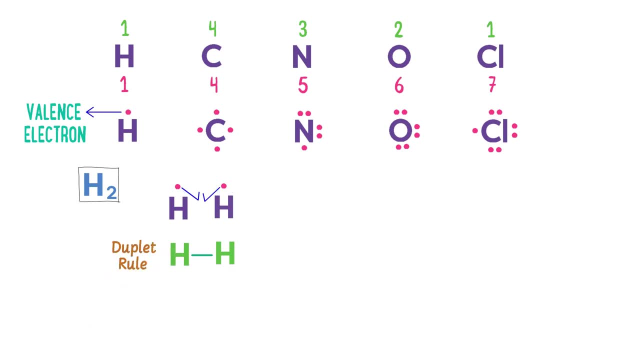 by both hydrogen atoms. Hence duplicate rule of both hydrogen atoms is completed. This is the Lewis structure of hydrogen molecule. This single bond represents two electrons or one pair of shared electrons. Hence noted down, this Lewis structure of hydrogen. Secondly, consider oxygen molecule. I take 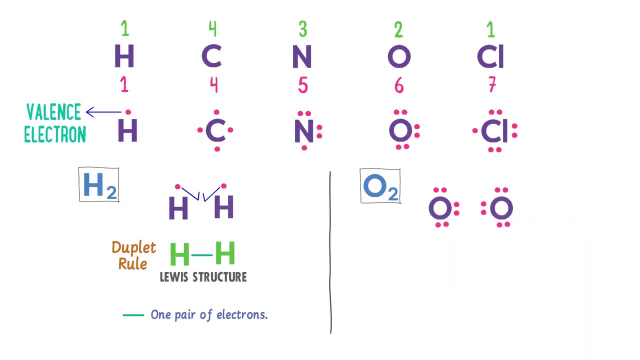 two atoms of oxygen. There are already six electrons present in the valence shell of this and this oxygen atom, So they will share two electrons each in order to complete their octet rule and we get this structure. Remember that double bonds represents four electrons, are two pairs of shared electrons, These two dotted. 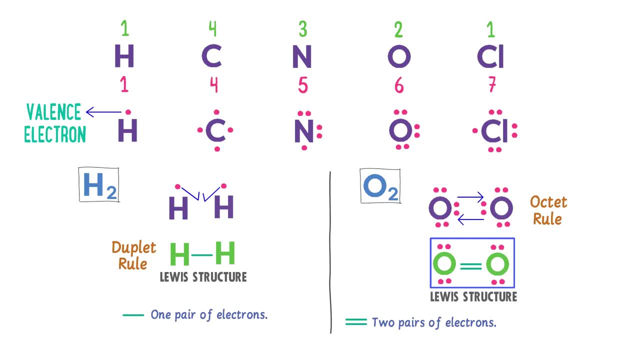 pair of electrons on this oxygen atom and on this oxygen atom are called lone pairs of electrons. They are called lone pairs because they do not participate in chemical bonding. Thus this is the Lewis structure of oxygen molecule. Also noted down that in this case, half arrow represents the flow of only one electron. 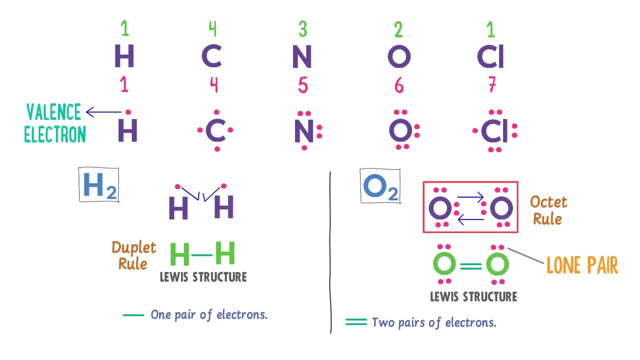 while in this case the full arrow represents the flow of two electrons. Thirdly, consider HCl. I take one atom of hydrogen in an electron and the next atom of hydrogen is a chemical bond. So this is hydrogen and one atom of chlorine. Hydrogen needs one more electron to complete its duplicate. 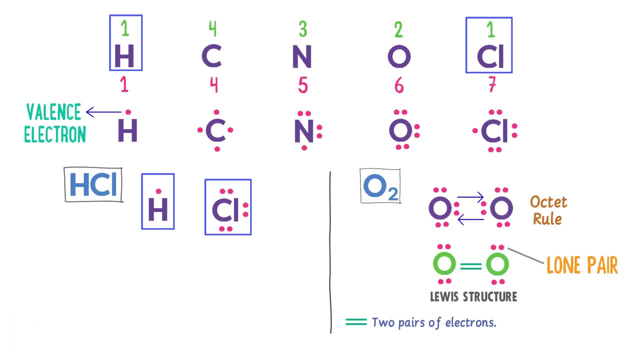 rule and chlorine also needs one more electron to complete its octet rule. So they mutually share a pair of electron and we get this structure. There are three lone pairs on chlorine, So this is the Lewis structure of HCl. Fourthly, consider CH4. I take one atom of carbon and four atoms of hydrogen. We know. 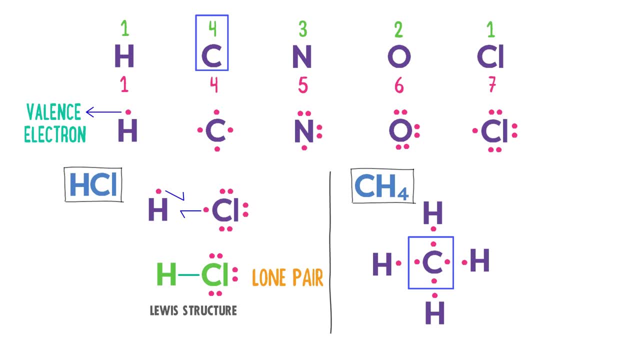 that carbon needs four more electrons to complete its octet rule, while hydrogen atoms need one electron each to complete its duplicate rule. So each hydrogen atom shares its one electron with carbon And carbon share its four electrons with each hydrogen atom and we get this structure. 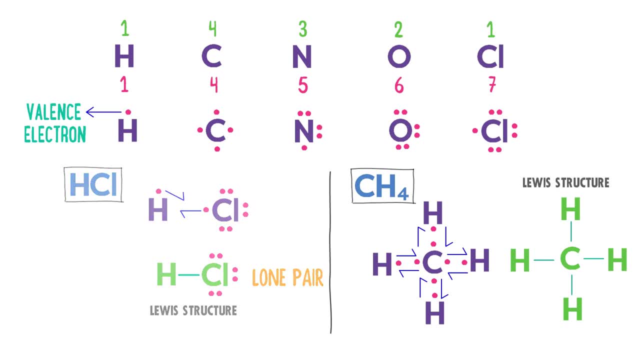 Thus, this is the Lewis structure of CH4.. Fifthly, consider NH3. I take one atom of nitrogen and three atoms of hydrogen. We know that nitrogen needs three more electrons to complete its octet rule and hydrogen atoms need one electron each to complete its duplicate rule. Nitrogen shares its three electrons. 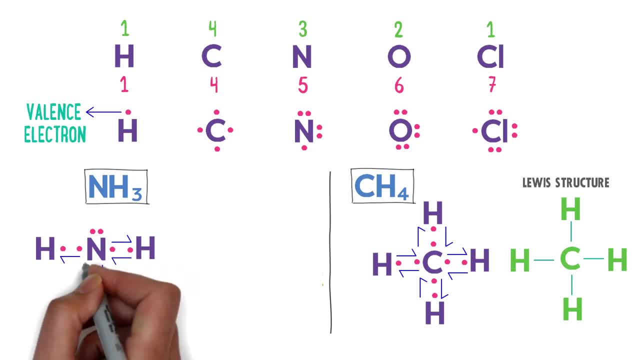 with hydrogen, and hydrogen atoms share one electron. with hydrogen, We get this structure. There is only one lone pair present on nitrogen atom. Thus this is the Lewis structure of NH3.. Finally, consider H2O. I take one atom of oxygen and two atoms of hydrogen. We know that oxygen needs two more electrons to complete its octet rule and hydrogen atoms need one electron each to complete its duplicate rule. And hydrogen atoms need one electron each to complete their doublet rule. thus oxygen atom shares its two electrons with each hydrogen atom and hydrogen atom shares one electron each with oxygen atom, and we get this structure.